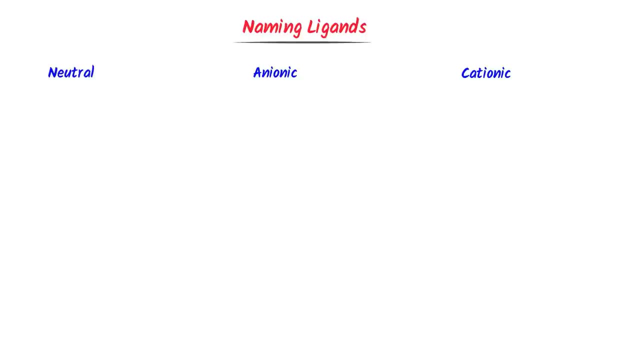 In case of neutral ligands, remember the names of these common ligands like ammonia, NH3, aqua, H2O, carbonyl CO, nitrosyl, NO, thiocarbonyl, CS, etc. In case of anionic ligands, the ID. 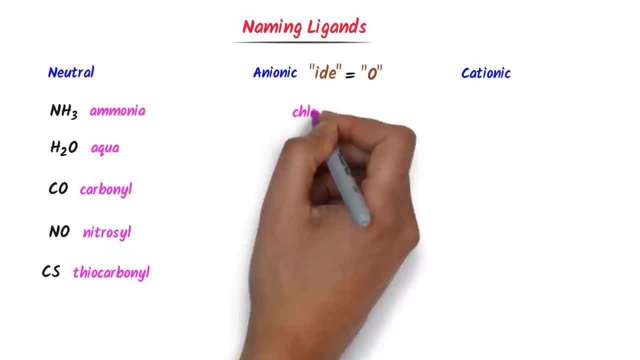 is replaced by O. Like chloride is written as chloro bromo, Br, hydro sulfito, SO, amido NH2, amido NH, isido N and oxo O, etc. In case of cationic ligands, we usually add IUM at the end. 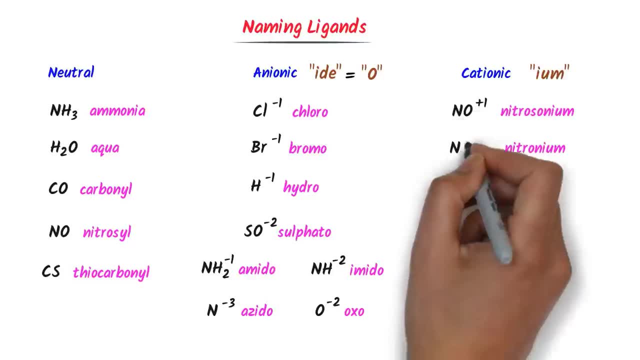 Like nitrosonium, NO, nitronium, NO2, hydrazinium, etc. Remember that ammonium ion NH4 is not a ligand because it has no lone pair. Thus remember these names of the ligands. Now we will learn. IUPAC nomenclature of ligands. 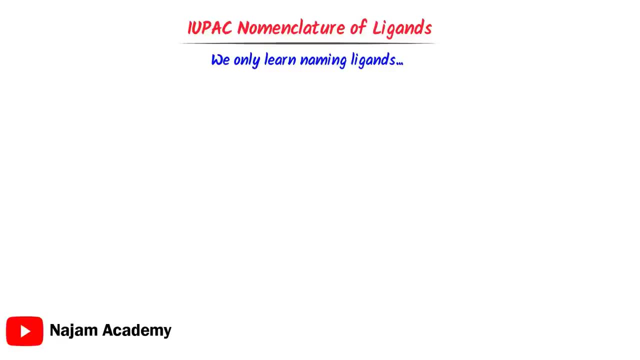 We will only learn naming ligands, because it will make things super easy. For example, consider these coordination compounds. We know that this is the coordination sphere. This is the ligand, cyanide, And this 6 means 6-cyanide ions. Now for this 6, I write hexa. 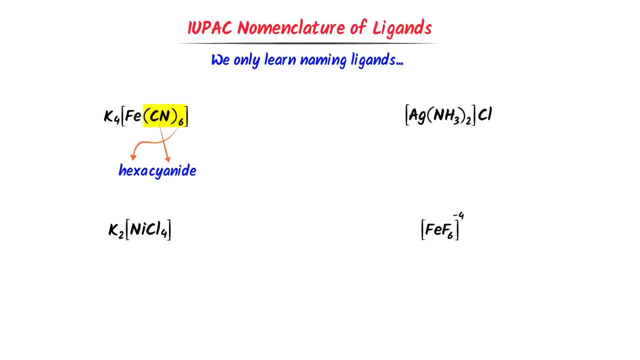 This is cyanide ligand. We know that for negative ligand we remove the IDE and we replace it by O, Thus I get hexa-cyano. Secondly, in case of this coordination compound, the ligand is ammonia NH3.. For this 2, I write di, And for this ammonia I write amine. Thus: 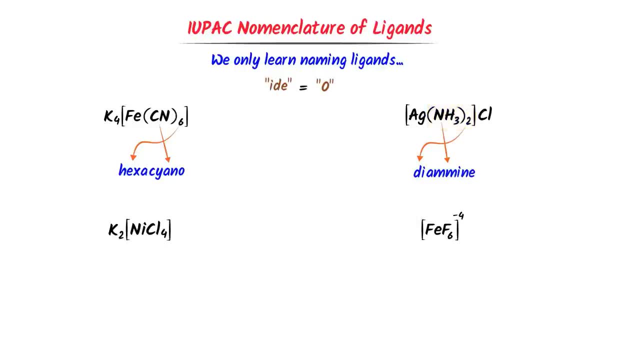 I get diamine. Thirdly, in case of this coordination compound, the ligand is chlorine And there are 4 ions of chlorine. I write tetra. For chlorine ion, I write chloro, Thus I get tetrachloro. Fourthly, in case of this coordination compound, the ligand is fluorine And there are 6. 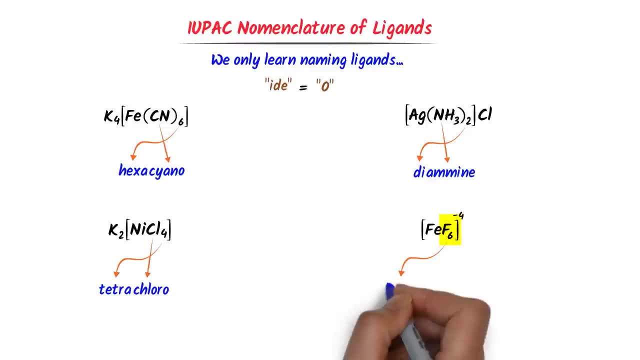 ions of fluorine. For this 6, I write hexa. For the fluorine ion, I write fluoro, Thus I get hexafluoro. Hence noted down these 4 examples. Now consider these coordination compounds. 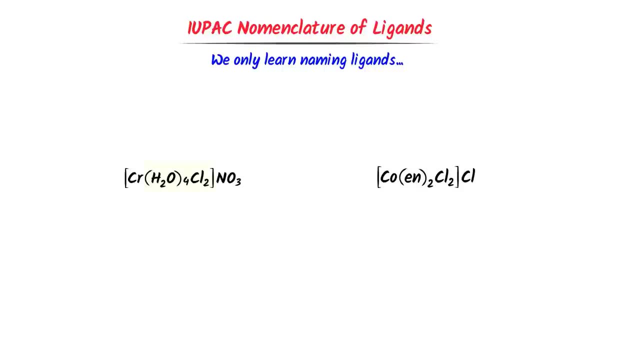 In case of this coordination compound, this is C, This is Ss. Thus we know that these ions are l-oxydechloro and manganese, whatever. Now we will learn. IUPAC nomenclature of five governments compound. there are two ligands: One is chlorine and the other is water, H2O. We know that water. 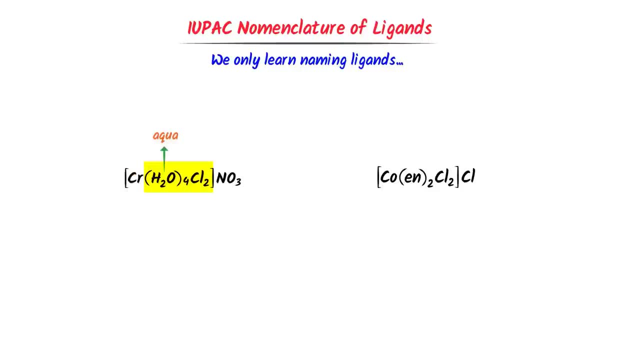 is a neutral ligand and its name is aqua. While chlorine is an ionic ligand, we write chloro for it. Now listen carefully. If there are two or more ligands, we write them in alphabetic order. Let me repeat it: If there are two or more ligands, we write them in. 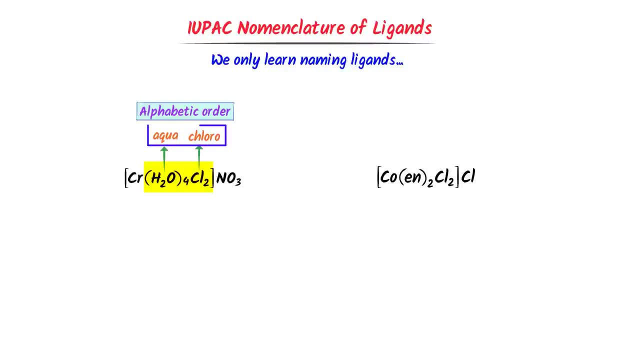 alphabetic order. We know that A comes first, then C, So I write aqua and then chloro. We know that there are four molecules of water. I write tetraaqua. Well, there are two ions of chlorine. I write dichloro. Remember that there is a chlorine in the water. So I write. 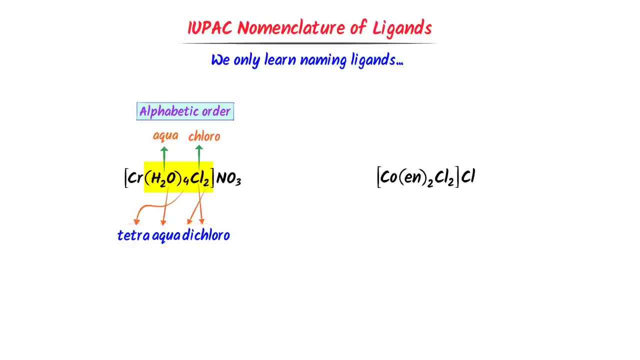 dichloro. Remember that there is a chlorine in the water, So I write dichloro. Remember that there is a chlorine in the water, So I write dichloro. Remember that there is no space while writing names of ligands, Thus I get tetraaqua dichloro. Secondly, in case 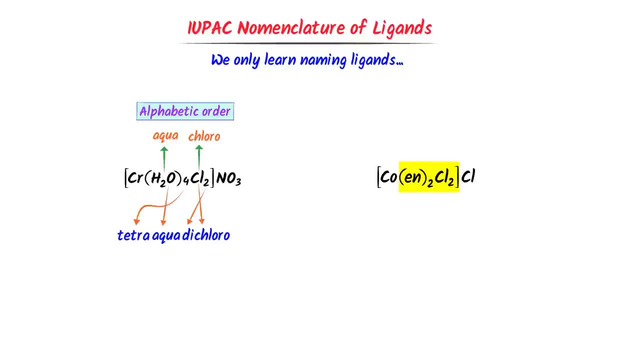 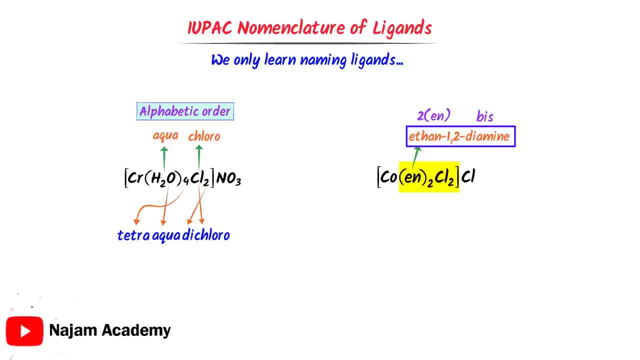 write die, because die is already there, and diamine. If there are three En molecules, we write trace. If there are four En molecules, we write tetra case and so on, According to the rule C, and chloro comes first, then En-ethane-1-2-diamine. So I write chloro and then I write ethane-1-2-diamine. 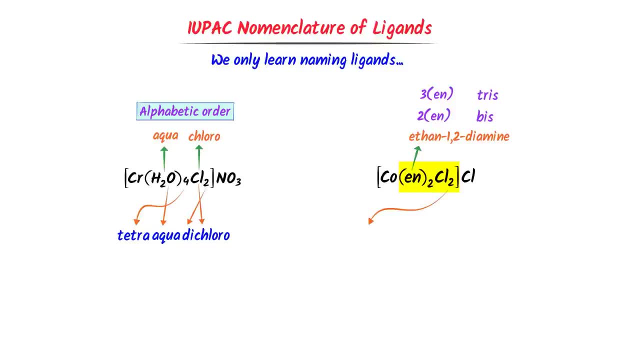 There are two chlorine ions, I write dichloro. There are two En molecules: I write base-ethane-1-2-diamine. Remember that there is no space between the words. Thus I get dichloro-base-ethane-1-2-diamine. 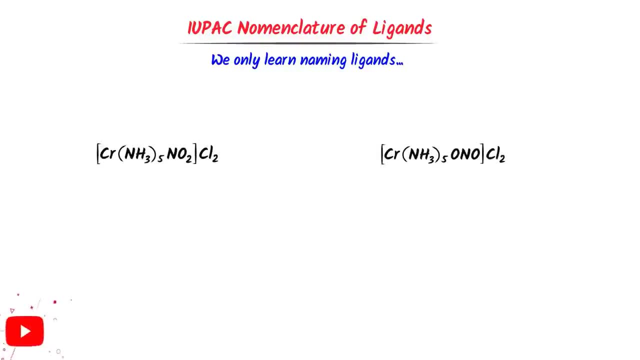 Now consider these coordination compounds. In this case there are two ligands, NH3 and No2.. Remember that this No2 is known as nitrate-2-N. According to alphabetic order, ammonia is written first, then nitrate-2-N. There are five molecules of ammonia I write. 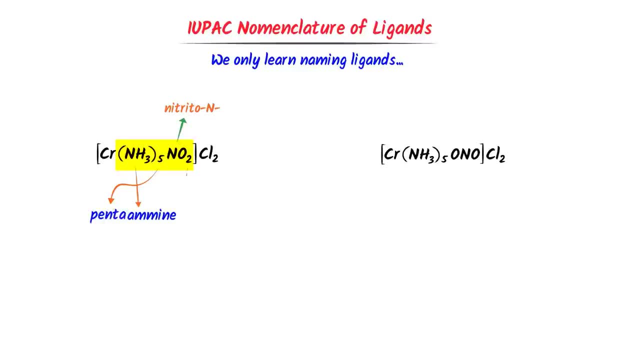 pentamide For the NO2, I write nitrate to N. Thus I get pentamine nitrate to N. Secondly, in this coordination compound there are also two ligands, NH3 and NO. Remember that this NO is known as nitrate to O. 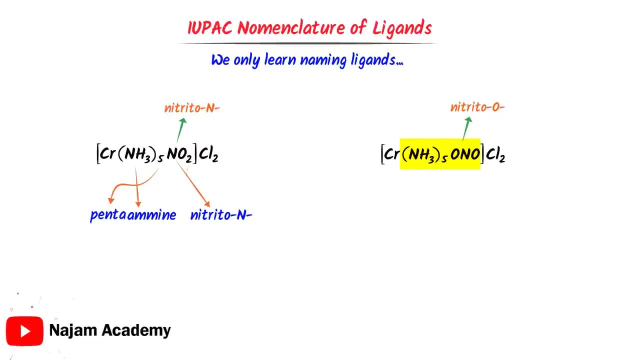 According to the alphabetic order, there are five molecules of NH3.. I write pentamine For this. NO, I write nitrate to O. Thus I get pentamine, nitrate to O. Therefore, using this simple method, we can easily name ligands of coordination compounds. 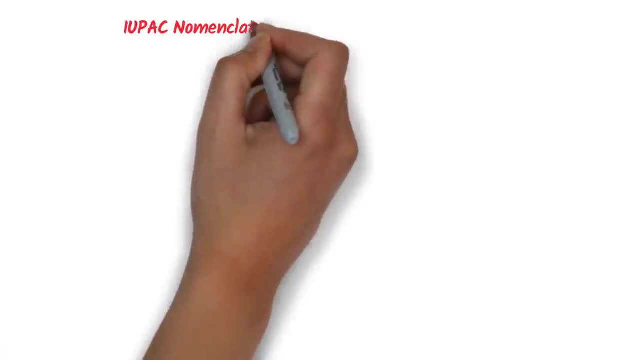 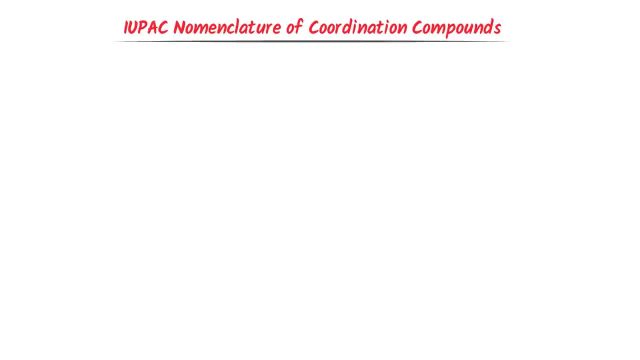 Hence note it down. Now we will learn IUPAC nomenclature of coordination compounds. Well, I will follow these steps. First, we will learn the nomenclature of coordination compounds. We will name coordination compounds from left to the right. 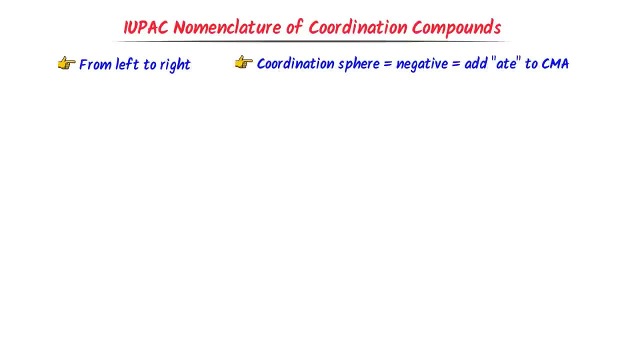 Secondly, if the coordination sphere is negative, we will add ATA to the central metal atom. Now consider these coordination compounds. We know that the left side of the coordination compound is always positive and the right side of the coordination compound is always negative. 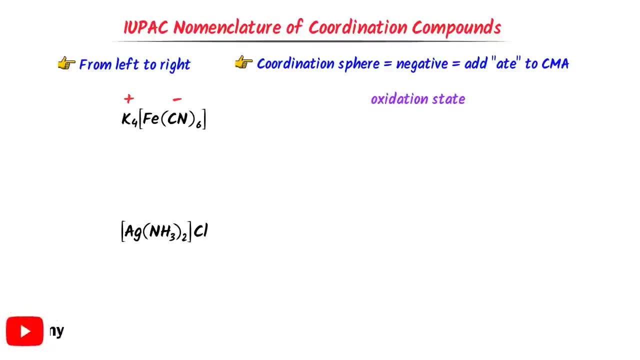 Firstly, I will find the oxidation state of central metal atom. I write: 4 potassium plus iron plus 6 cyanide ions is equal to zero, because the overall charge on this coordination compound is zero. We know that the oxidation state of potassium is positive: 1 and that of cyanide ion is negative. 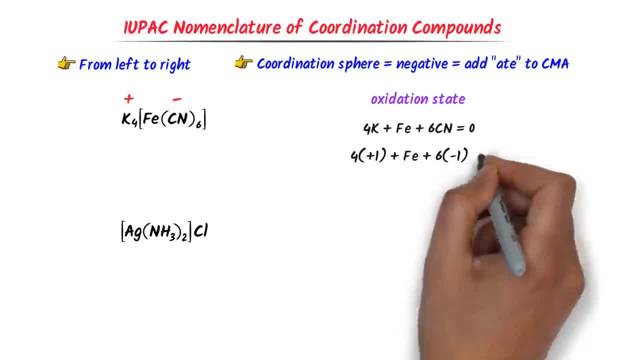 1. I write 4 into 1, plus iron plus 6 into negative: 1 equals to zero. After calculation, I write 4 into 1 plus iron plus 6 into negative: 1 equals to zero. After calculation I get iron is equal to positive 2.. 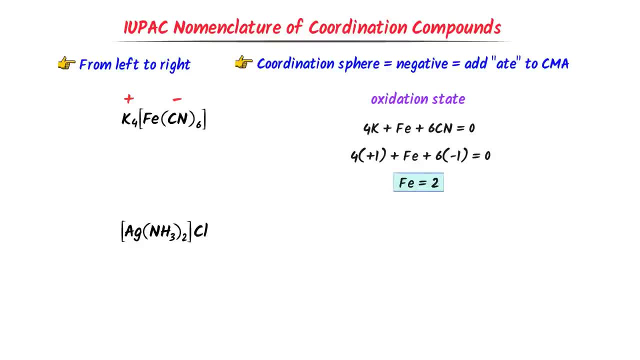 Hence the oxidation state of iron is positive. 2. Remember that if you do not know calculating oxidation state, then watch our lecture and its link is given in the description. Now I write potassium. Remember that in case of counter iron, we do not consider the numbers. I mean do not. 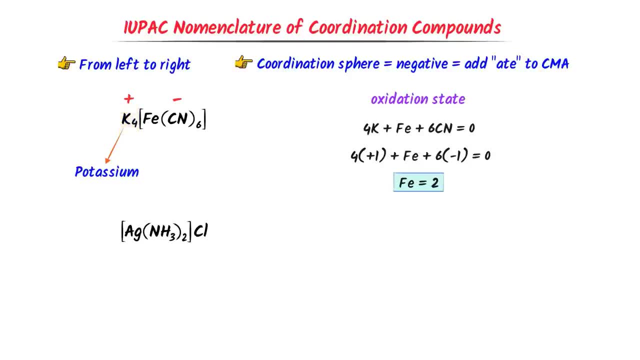 trite, di tri, etc. Secondly, in the coordination sphere, I name the ligand And there are six ions of cyanide. I write hexacyno. Lastly, the central metal atom is iron. We know that if the coordination sphere has negative charge, we put Ate with the central metal atom. Let 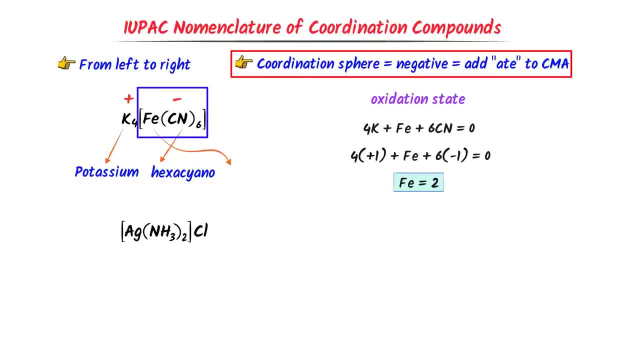 me repeat it: If the coordination sphere has negative charge, we put Ate with the central metal atom. So for this iron I write ferrate. The oxidation number of iron is 2.. I write here 2.. Thus I get potassium hexacynoferrate 2.. So this is the IUPAC name of this coordination. 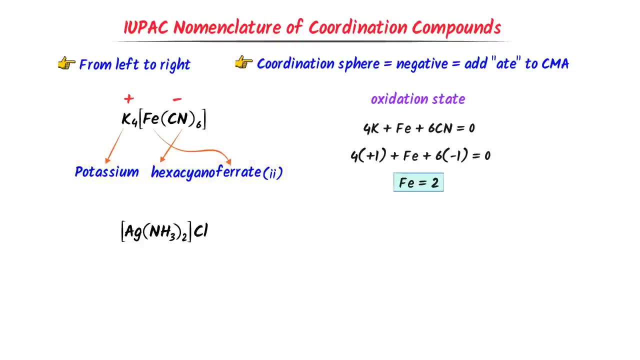 compound. Now, in this case, as usual, I write here positive charge and I write here negative charge. Here I will find the oxidation number of central metal atom, which is silver. I write silver plus 2. ammonia plus chlorine ion equals to zero. We know that, the oxidation state of ammonia being a neutral, 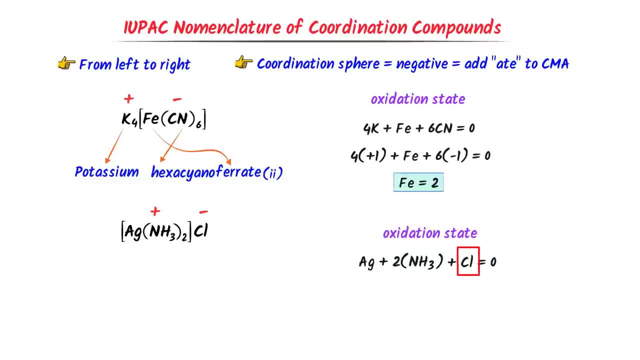 molecule is zero and that of chlorine ion is negative one. I write silver plus 2 N to zero. plus negative one is equal to zero. After calculation I get silver is equal to one. Hence the oxidation state of central metal atom, silver, is one According to the rule. 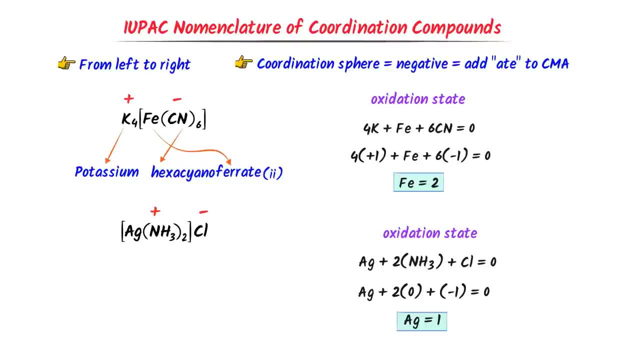 I firstly name the ligand In the coordination sphere. the ligand is ammonia and there are two molecules of ammonia. I write diamine And in this situation the silver is two molecules. I write thiamine For this silver. I write thiamine And for this silver I. 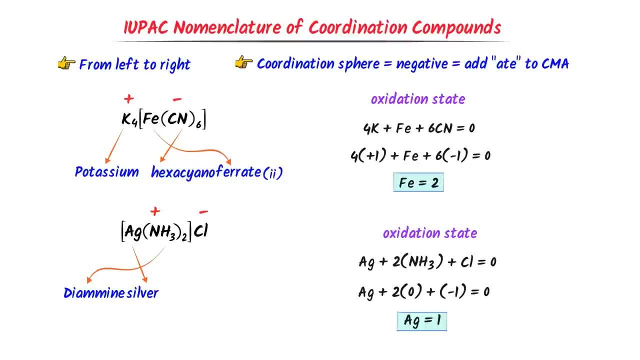 write thiamine And the corresponding number of lisium. i, I write thiamine. Even with thiamine, I write silver. Remember that the coordination sphere has positive charge, So I do not put A-T-E with the central metal atom. We know that the oxidation state of silver is 1.. I write here: 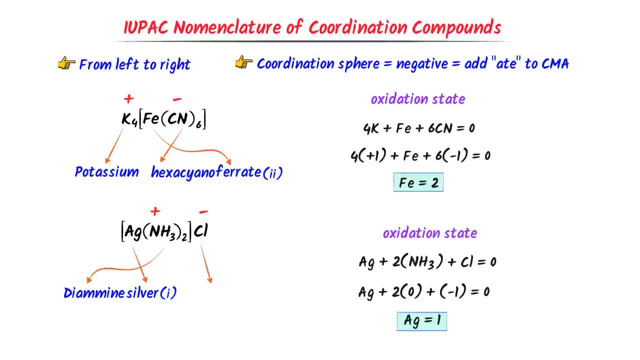 1. For this chlorine I just write chloride, Thus I get diamine silver 1 chloride. Hence this is the IUPAC name of this coordination compound. Now consider these coordination compounds. As usual, I write here positive charge and I write here negative charge. 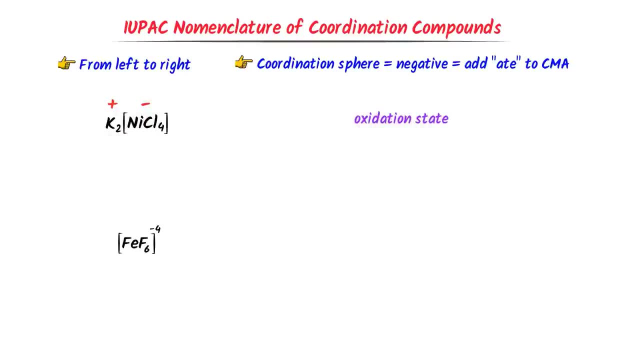 Secondly, I calculate the oxidation state of central metal atom, which is nickel. After calculation I get: the oxidation state of nickel is positive, 2.. According to the rule, I write potassium And the coordination sphere. there are four ions of chlorine. I write tetrachloro, The central. 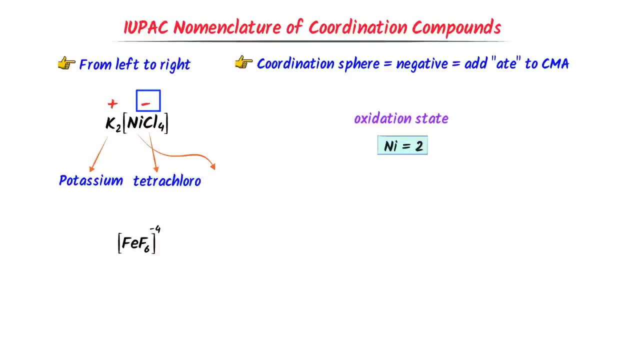 metal atom is nickel And the charge on coordination sphere is negative. Hence I write nickelate. The oxidation state of nickel is 2.. Thus I get potassium tetrachloro nickelate 2.. Hence this is the IUPAC name of this coordination compound. 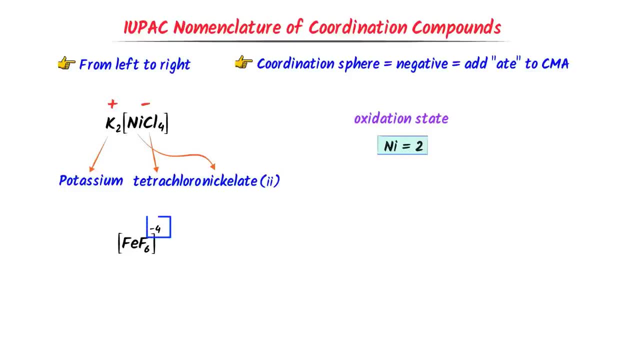 In case of this coordination compound, I write nickel, Hence I get potassium tetrachloro, nickelate 2. So I do not put any charge on it. What about the oxidation state? Well, after calculation, I get the oxidation state of: 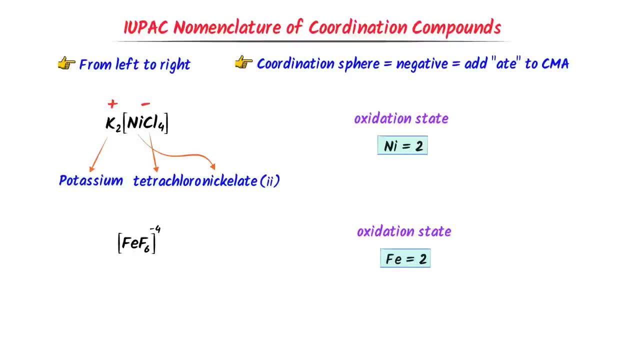 iron is positive 2.. Hence the oxidation state of iron is positive, 2.. Now in the coordination sphere there are six fluorine ions. I write here hexa, And we know that the ligand is fluorine. I write fluorine. The central metal atom is iron. We can see that the charge on coordination 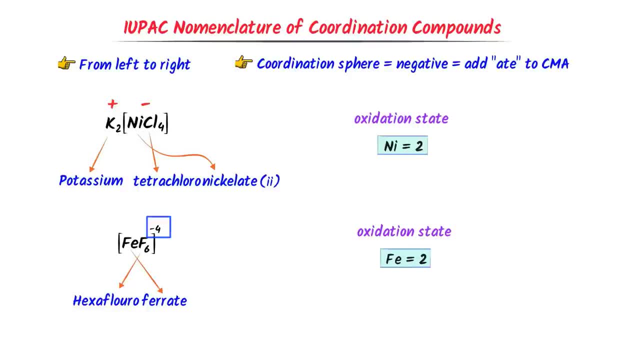 sphere is negative, I write ferrite. The oxidation state of iron is positive, 2. I write here 2. Thus I get hexafluoroferrite 2-ion. Hence, this is the IUPAC name of this coordination. 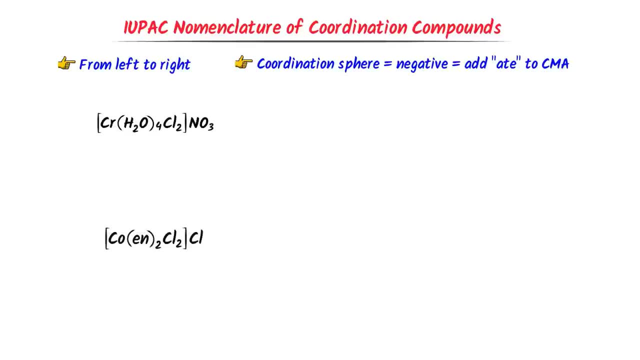 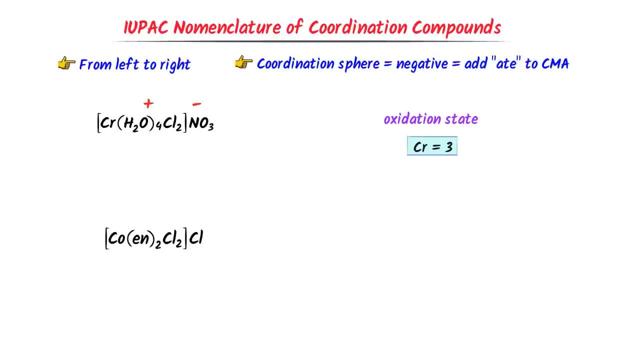 of chromium is 3.. In the coordination sphere there are two ligands: water and chlorine ion. According to the alphabetic order, I write firstly aqua and then chloro. There are four molecules of water. I write tetraaqua: There are two molecules of chlorine. 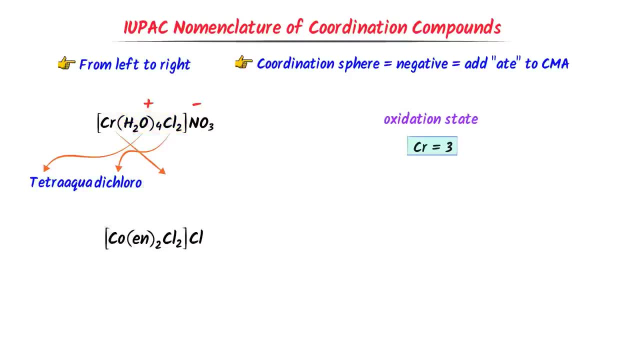 I write dichloro. The central metal atom is chromium. The charge on coordination sphere is positive, Hence I only write chromium. The oxidation state of chromium is 3.. For this NO3, I write nitrate. Thus I get tetraaqua, dichlorochromium nitrate. Hence this is the 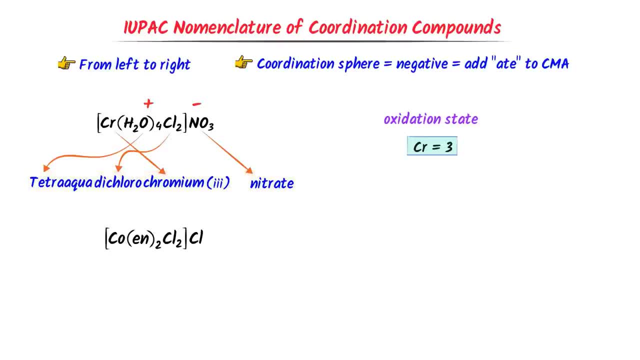 IUPAC name of this coordination compound. Now, in case of this coordination compound, I write positive charge and negative charge. The oxidation state of cobalt is 3.. Here in the coordination sphere there are two ligands, en and chlorine. According to the rule for these two chlorine ions, I write: 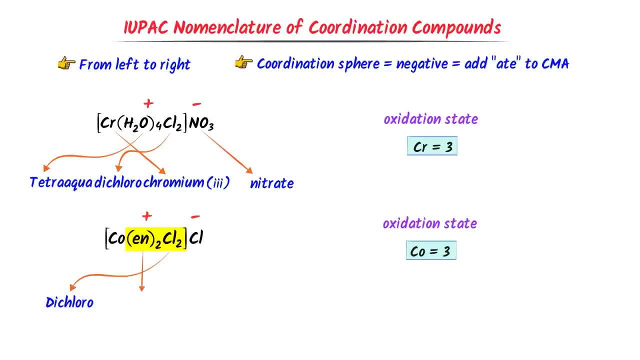 dichloro. For these two en molecule, I write bisethane 1,2-diamine. Now, in case of this coordination compound, I write positive charge and negative charge. Hence I write positive charge and negative charge. For the central metal atom, I write only cobalt. The oxidation state of cobalt is 3.. For this, 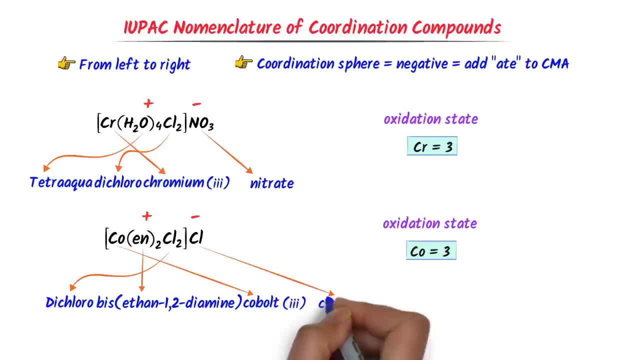 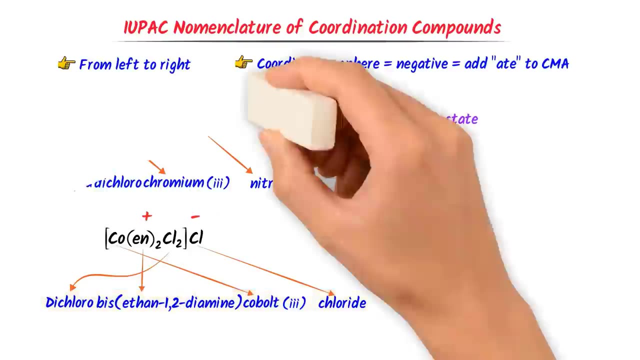 chlorine. I just write chloride. Thus I get dichloro bisethane, 1,2-diamine, cobalt 3-chloride. Hence this is the IUPAC name of this coordination compound. Now consider this coordination compound. I write positive charge and negative charge. 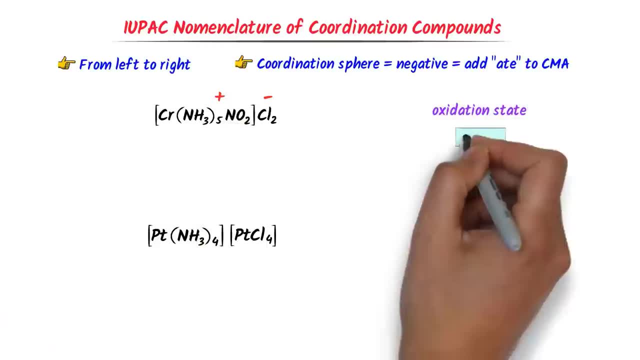 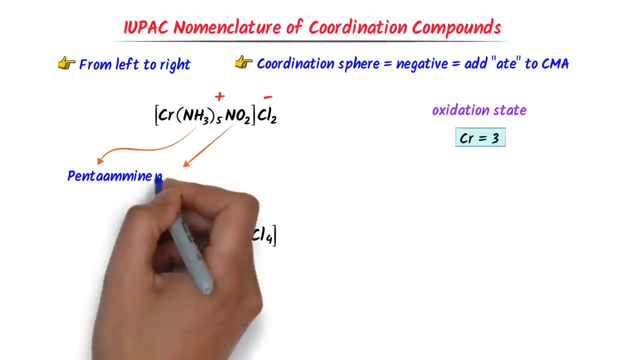 and negative charge. The oxidation state of chromium is 3.. I write pentaamine For this NO2,. I write nitrate 2N For this chromium. I write chromium And the oxidation state of chromium is 3.. For this chlorine I just tried chloride. Thus I get pentaamine nitrate 2N, chromium 3, chloride. 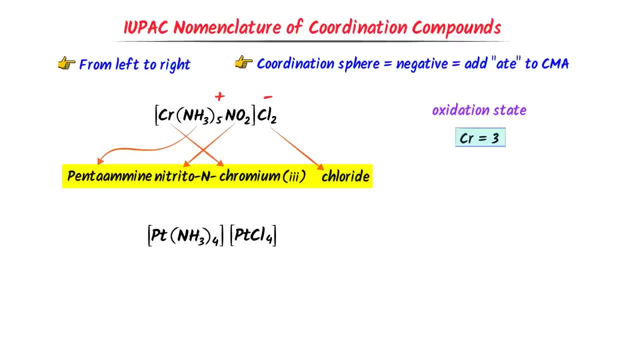 Hence this is the IUPAC name of this coordination compound. Now consider this coordination compound. I write positive and negative charge. The oxidation state of platinum and this coordination sphere is 2.. While the oxidation state of platinum and this coordination sphere is also 2.. Now for these four molecules of NH3, I write tetraamine. 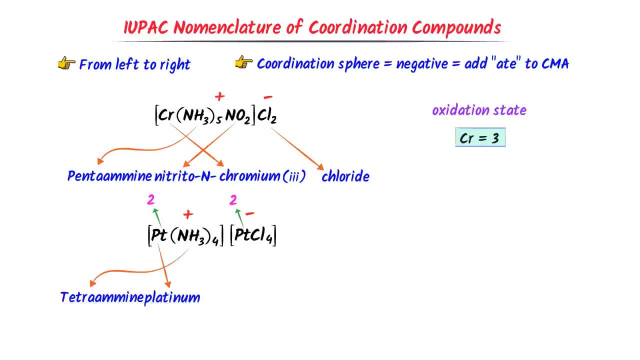 For platinum, I write tetraamine, I write tetraamine. For octane, I write tetraamine- platinum. The oxidation state of platinum is 2.. Secondly, for these four ions of chlorine, I write tetrachloro. The charge on coordination sphere is negative. For this platinum, I write 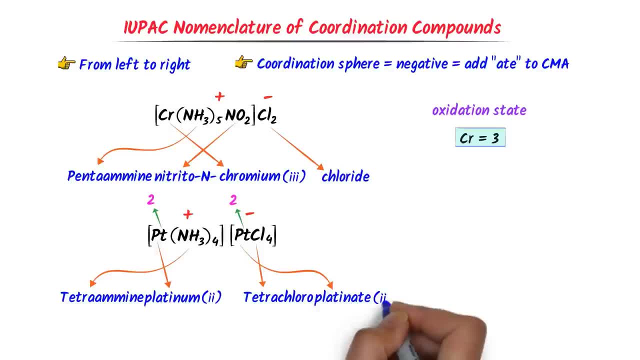 platinet. The oxidation state of platinum is 2.. Thus I get tetraamine platinum 2, tetrachloro platinet 2.. Hence this is the IUPAC name of this coordination compound. 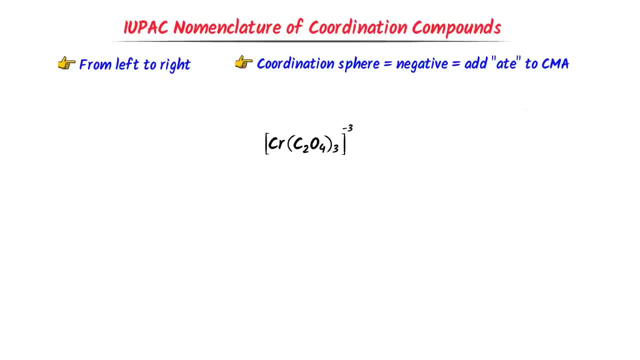 Finally, consider this coordination compound. Pause the video and try to write its IUPAC name. Well, there is already negative charge present on it. The oxidation state of chromium is 3.. Remember that C2O4 is a ligand which is known as oxyleto. 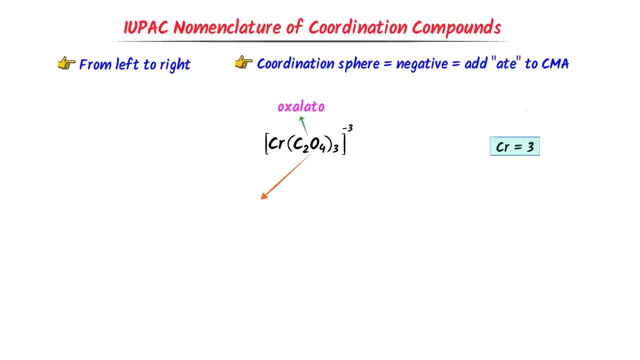 We can consider the oxidation firm of C2O4 as a log. see that there are three oxalates. I write trioxalato. the central metal atom is chromium and the charge on coordination sphere is negative. I write chromate: the oxidation.